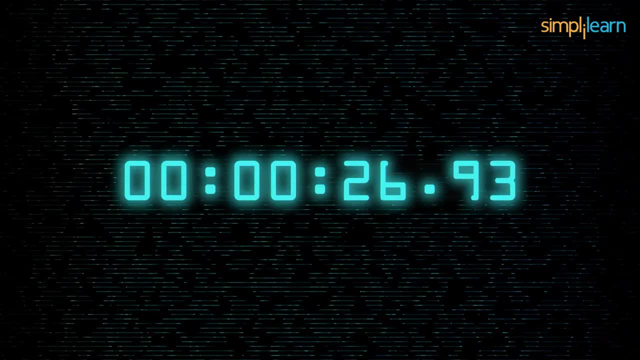 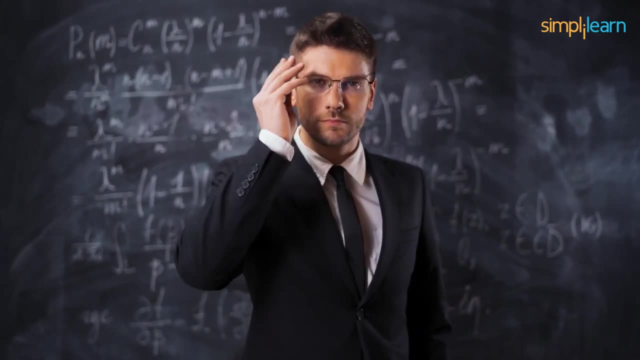 Finally, we will touch upon time series analysis, a vital skill for data analysis. We will also cover sampling techniques, regression analysis and hypothesis testing, which are important skills for analyzing and forecasting data collected over time. By the end of this tutorial, you will have a solid foundation in these 10 key statistical 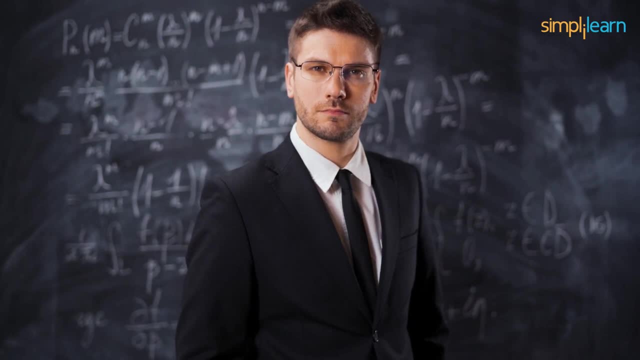 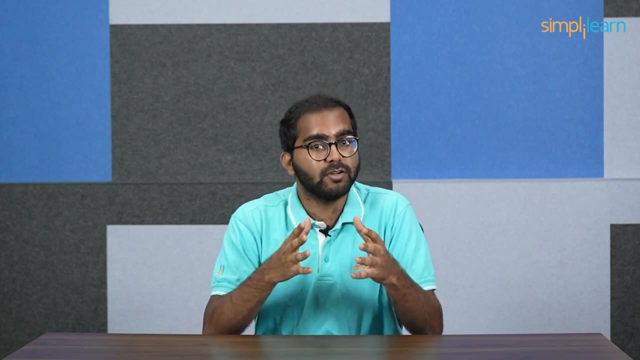 concepts empowering you to confidently embark on your data science journey. So let's dive in and unlock the power of statistics in data science. But before we get started, if these are the types of videos you'd like to watch, then you know how the YouTube algorithm works. 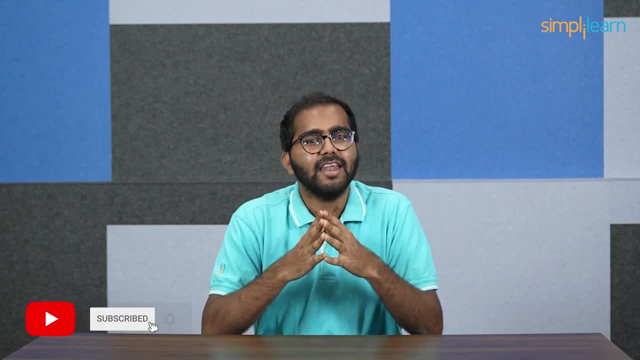 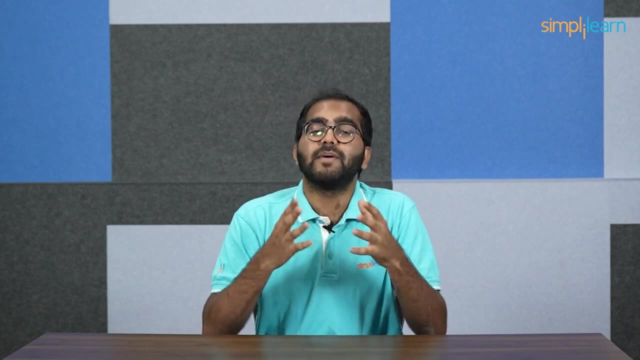 Let's do the drill: Get subscribed to our YouTube channel, like our videos and hit the bell icon to never miss an update from Simply Learn. If you're one of the aspiring data scientists, look at this video. If you're a data scientist looking for online training, graduating from the best. 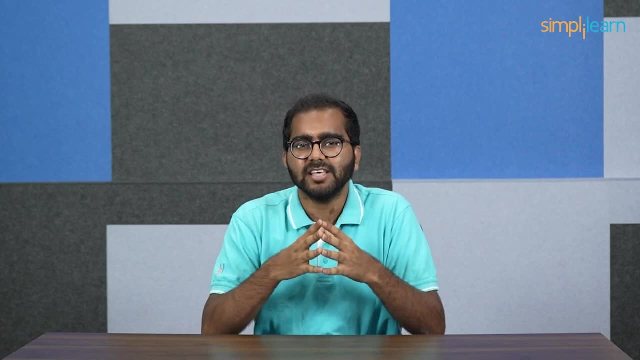 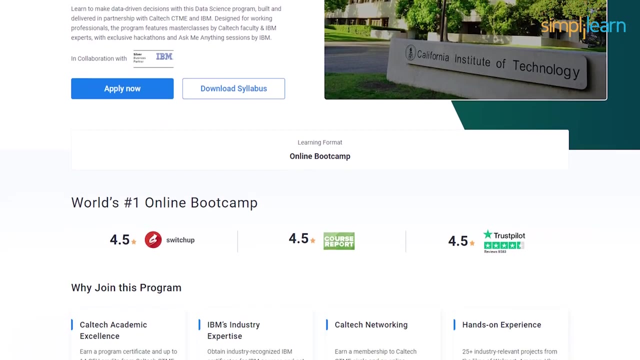 universities or a professional who elicits to switch careers with data science by learning from the experts, then try giving a shot to the Caltech postgraduate program in data science from Simply Learn in collaboration with IBM. The link in the description box should navigate to the homepage, where you can find a complete 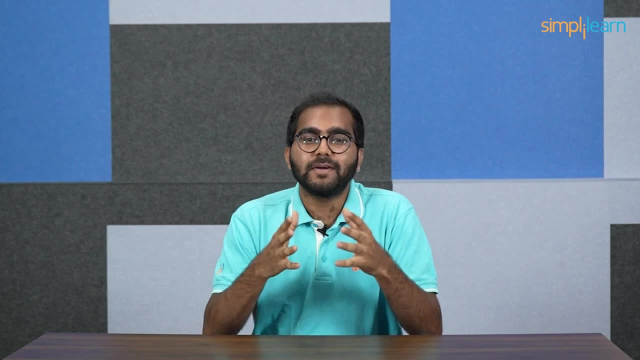 overview of the program being offered. Let's begin with discussing the top 10 most important statistics concepts for data science Over to our training experts. Hello all. Let's get started with the top 10 most important statistics concepts for data science. 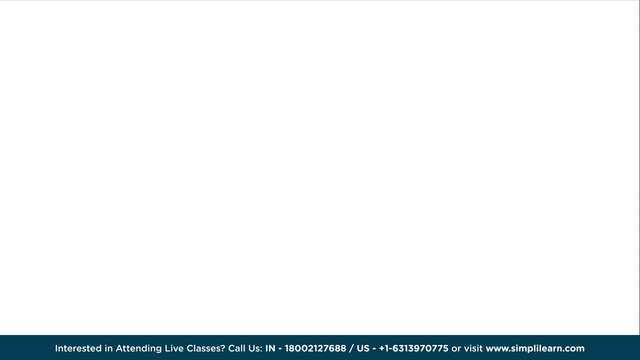 Hello all. Let's get started with the top 10 most important statistics concepts for data science. First on the list is descriptive statistics. Descriptive statistics involves summarizing and describing the main features of a dataset. It includes measuring, such as mean, median mode, standard deviation and range which 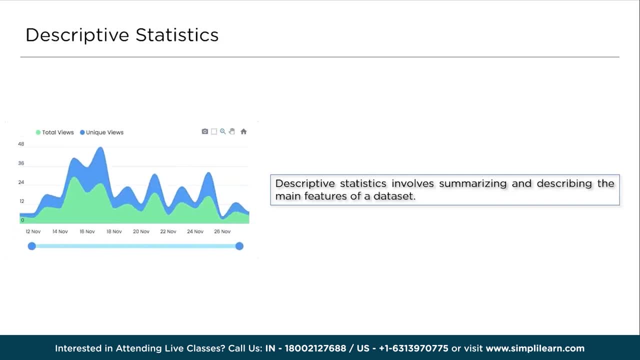 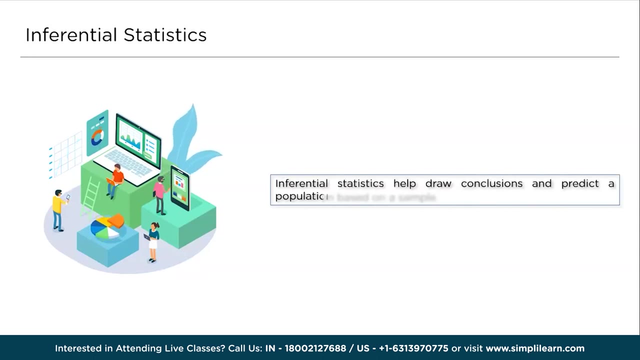 provide insights into the data's central tendency, spread and distribution. Now, proceeding ahead, we have inferential statistics. These statistics help draw conclusions and predict a population based on a sample. It involves hypothesis testing, confidence intervals and p-values, allowing data scientists 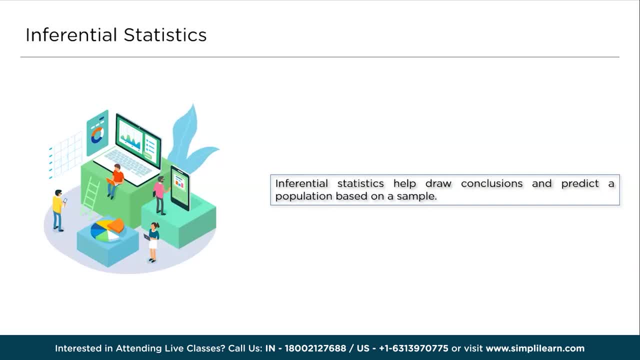 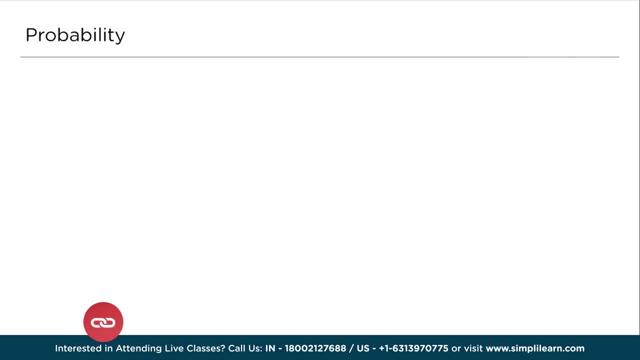 to make informed decisions and statements about the population from which the sample was drawn. Next on the docket is probability. Probability is the foundation of statistics. It measures the likelihood of an event occurring and enables data scientists to qualify uncertainty. Understanding probability is crucial. 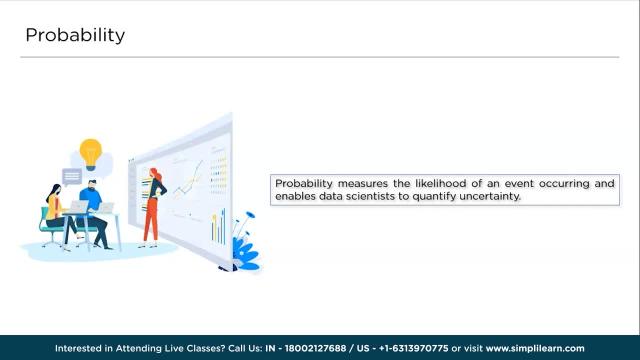 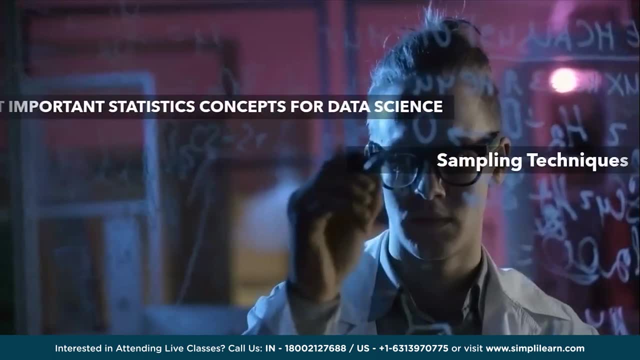 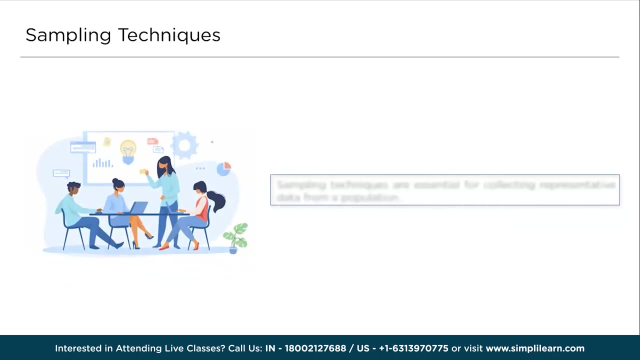 It is crucial for tasks such as estimating probabilities, calculating expected values and conducting Bayesian analysis. The fourth one on the list is sampling techniques. Sampling techniques are essential for collecting representative data from a population: Simple, random sampling, satisfied sampling, cluster sampling and systematic sampling. 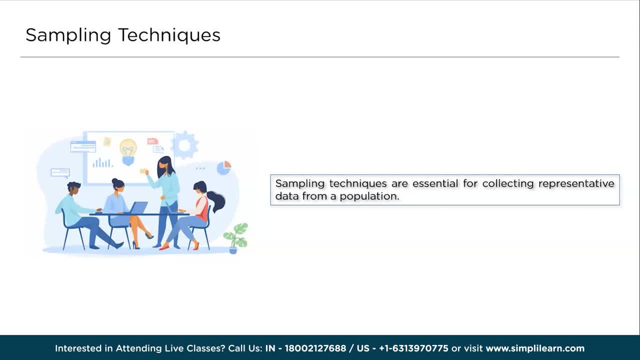 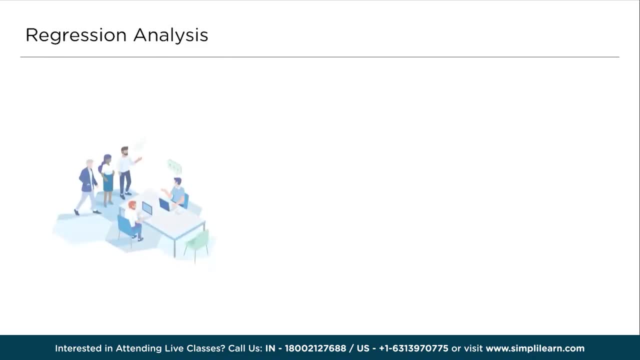 are standard techniques used to ensure that the sample accurately reflects the characteristics of population. Next on the docket is statistical statistics. These statistics can be used to determine the probability of a population being tested in the same way. The third one on the docket is regression analysis. 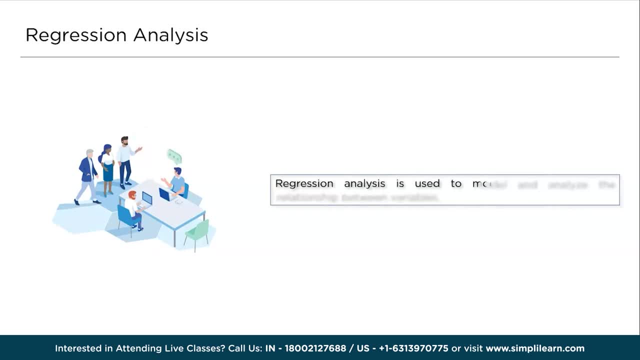 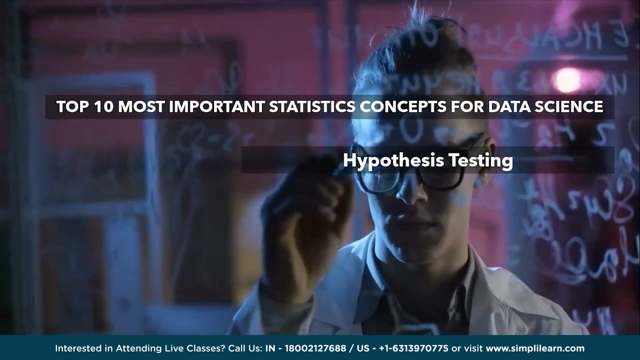 Regression analysis is used to model and analyze the relationship between variables. Simple, linear, multiple and logistic regression are commonly used techniques to understand how one or more variables influence an outcome or dependent variable. Proceeding ahead, we have hypothesis testing. Hypothesis testing is used to evaluate the validity of a claim or hypothesis about a 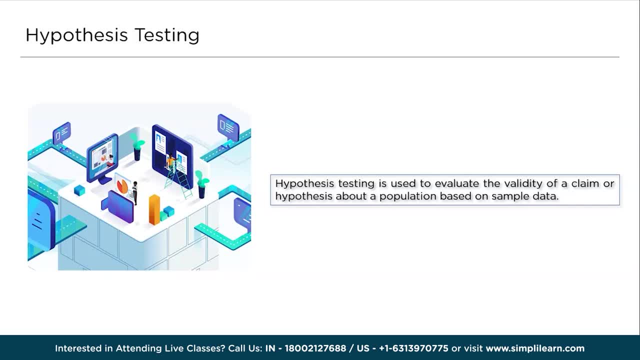 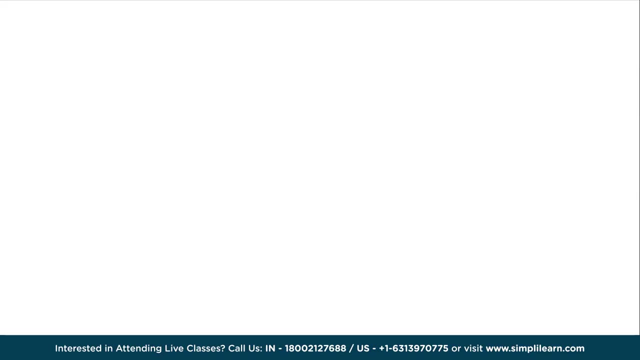 population based on sample data. It involves a number of parameters. It involves settling up a null and alternative hypothesis, calculating test statistics and make decisions based on p-values and significance levels. With that we can move on to the next one, that is, statistical distributions. 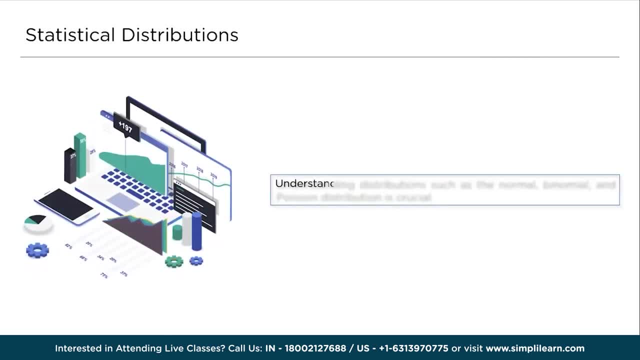 Statistical distributions describe data patterns and behavior. Understanding distributions such as the normal, binomial and Poisson distribution is crucial for analyzing and modeling various data types. Now we have the statistical distribution. We have the statistical inference in the eighth place. Statistical inference involves drawing conclusions and making predictions based on sample data. 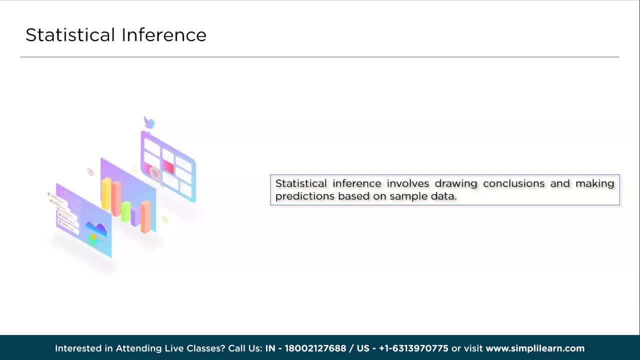 It includes concepts such as confident intervals, margin of error and sample size determination, which help quantify the precision and reliability of estimates and predictions. Proceeding to the ninth one, we have experimental design. Experimental design refers to the planning and structure of experiments to ensure valid 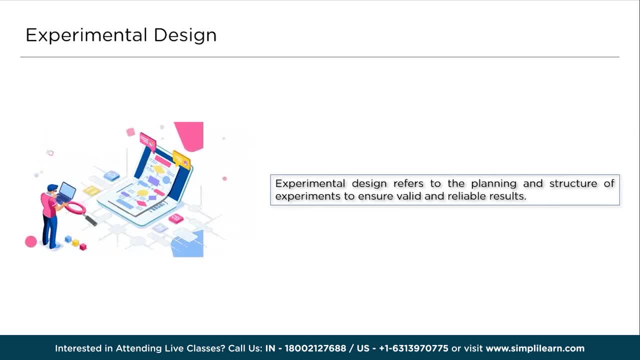 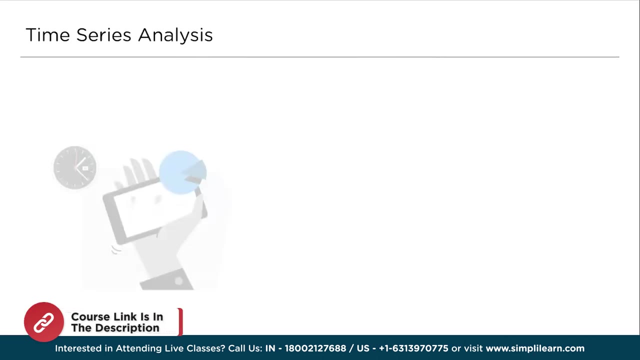 and reliable results. Concepts such as randomization, control groups and replication are used to minimize bias and co-founding variables, allowing data scientists to make casual inferences. Finally, we have the most important one, on the tenth place time series analysis.